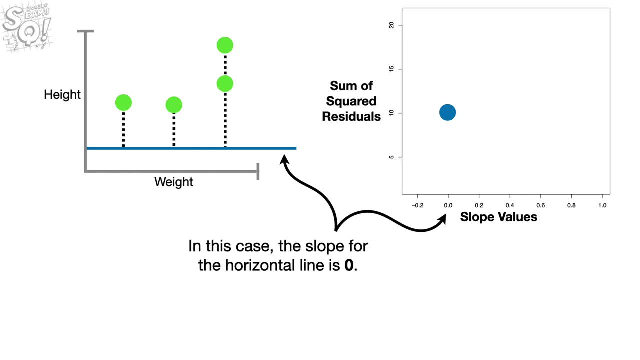 In this case, the slope for the horizontal line is zero. Now let's increase the slope to 0.2.. And calculate a new value for the sum of the squared residuals. Now let's increase the slope to 0.4.. And calculate a new value for the sum of the squared residuals. 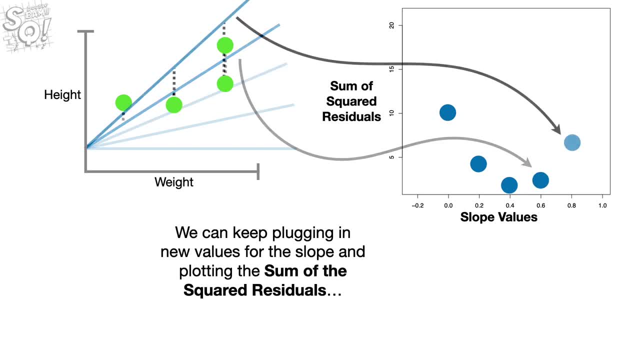 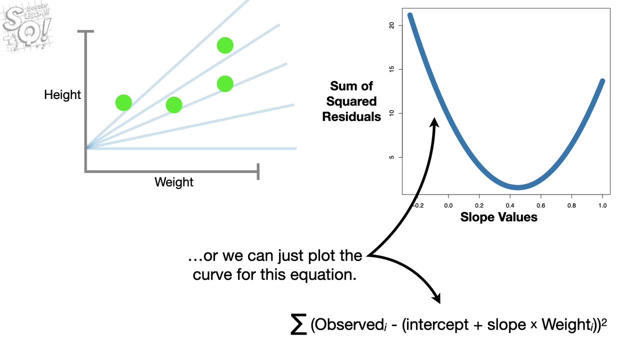 We can keep plugging in new values for the slope and plotting the sum of the squared residuals, Or we can just plot the curve for this equation. We can see that the best fitting line is at the bottom of the parabola. In other words, when the slope equals 0.45, we get the lowest sum of the squared residuals. 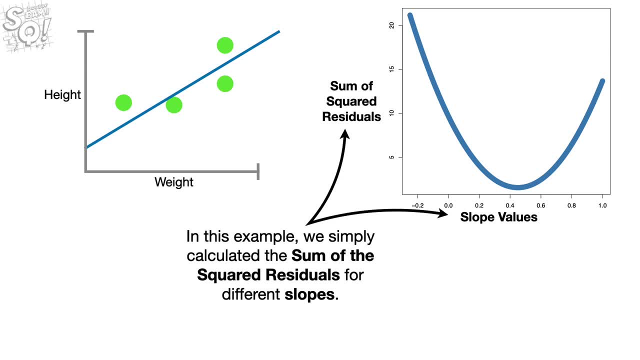 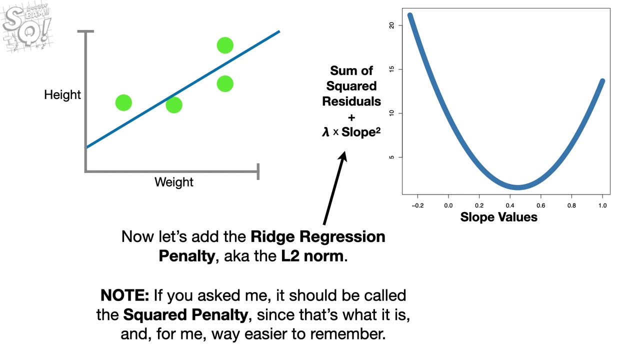 In this example, we simply calculated the sum of the squared residuals for different slopes. Now let's add the ridge regression penalty, aka the L2 norm. If you asked me, it should be called the squared penalty, since that's what it is. 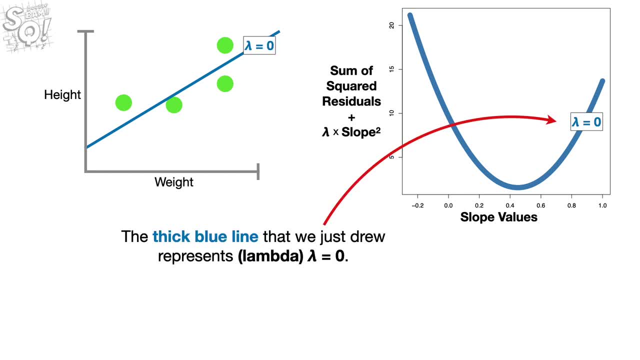 And for me way easier to remember. The thick blue line that we just drew represents lambda equals 0. This is because when lambda equals 0, the penalty is equal to 0. Regardless of the slope, And we are left with the original sum of squared residuals. 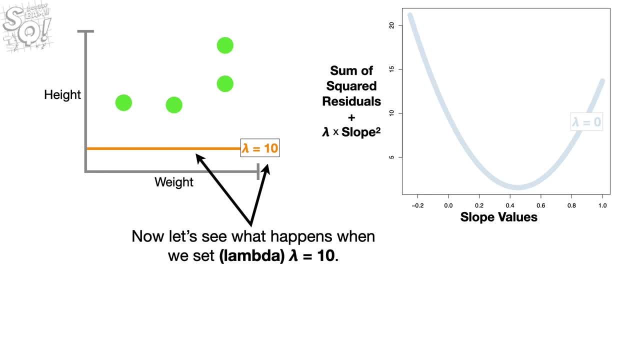 Now let's see what happens when we set lambda equal to 10.. And, just like before, we'll start with a horizontal line. Only this time the line is orange. Just like before, we can calculate the residuals, And we can calculate the sum of the squared residuals plus lambda times the slope squared. 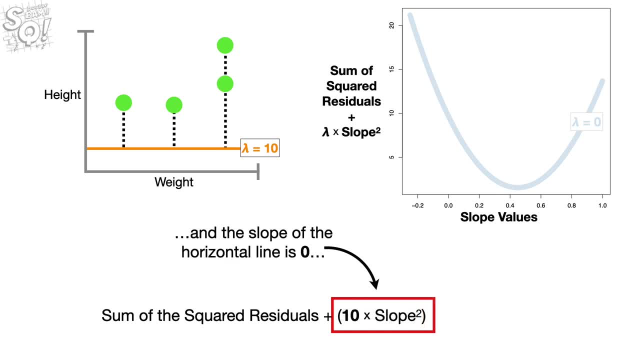 In this case, lambda equals 10.. And the slope of the horizontal line is 0.. So the penalty is 0.. So we plot the sum of the squared residuals here. Now let's increase the slope to 0.2.. Note: the residuals are smaller than before. so the sum of squared residuals is smaller than before. 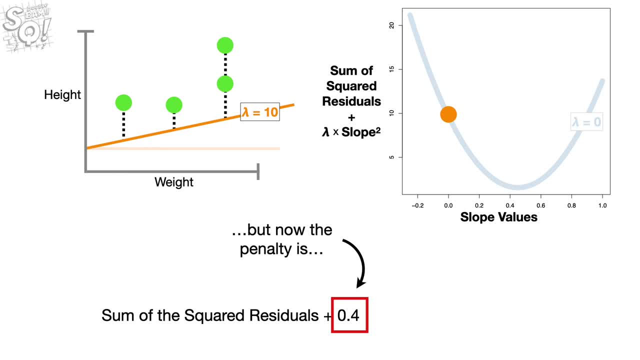 But now the penalty is 0.4.. And that gives us this point on the graph. Now let's increase the slope to 0.4.. And the residuals are even smaller. But now the penalty is 1.6.. And that gives us this point on the graph. 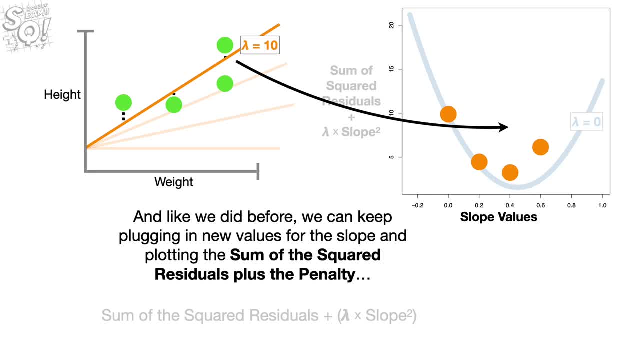 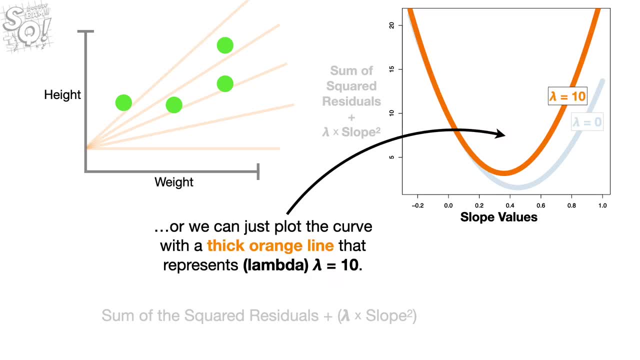 And, like we did before, we can keep plugging in new values for the slope and plotting the sum of the squared residuals plus the penalty. Or we can just plot the curve with a thick orange line that represents lambda equals 10. The bottom of the parabola is where the slope gives us the lowest sum of squared residuals plus penalty. 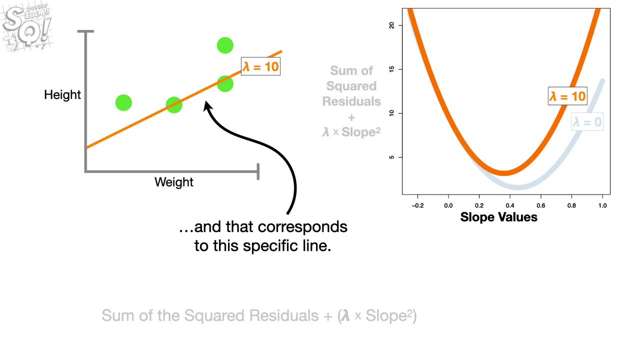 And that corresponds to this specific line. And when we compare that to the optimal slope when lambda equals 0, we see that setting lambda equal to 10 results in a smaller optimal slope. Note: we can also see that when lambda equals 10,. 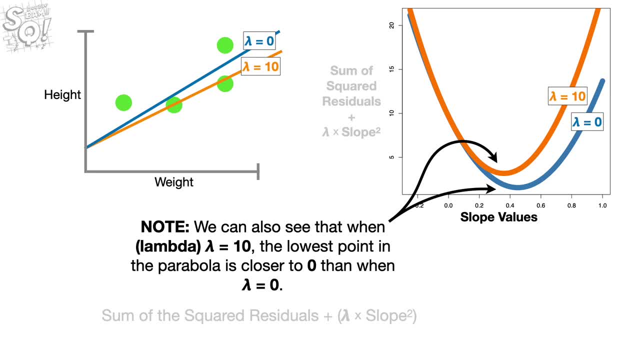 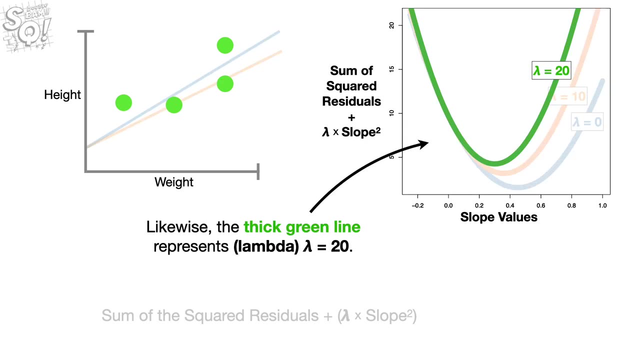 the lowest point in the parabola is closer to 0 than when lambda equals 0. So either way we look at it, we see that the larger value for lambda shrunk the optimal value for the slope. Likewise, the thick green line represents lambda equals 20.. 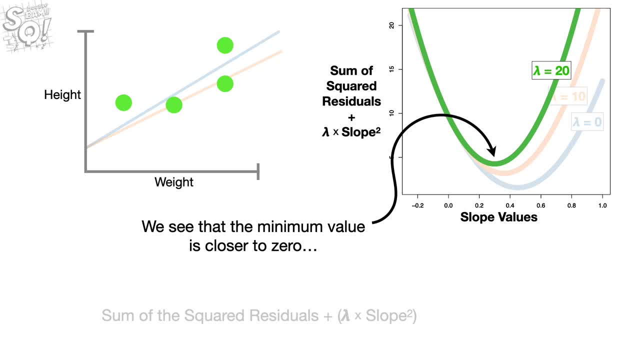 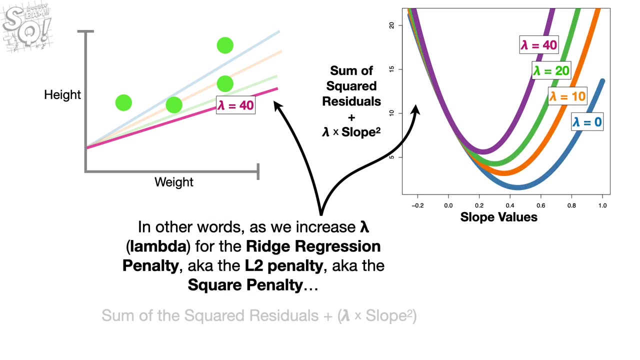 We see that the minimum value is closer to 0. And the optimal slope has shrunk some more. The purple lines represent lambda equals 40 and it shrinks the slope even more. In other words, as we increase lambda for the ridge regression penalty. 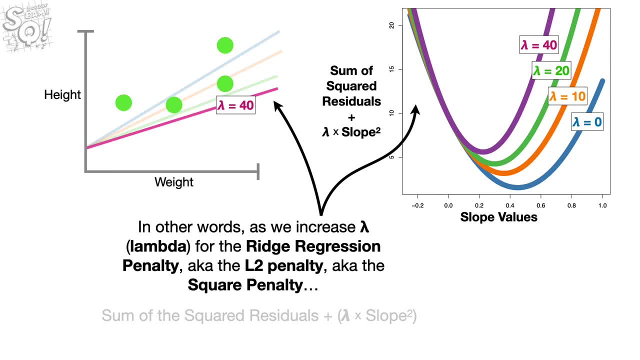 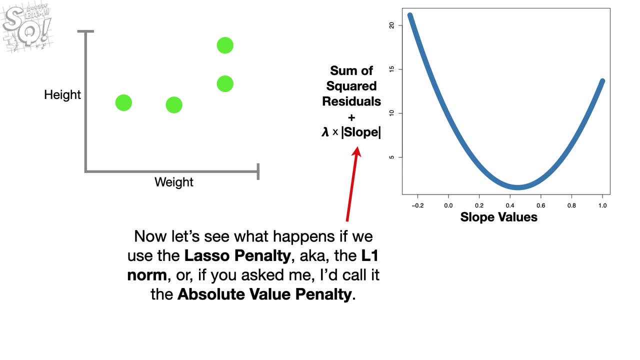 aka the L2 penalty, aka the square penalty. the optimal slope gets closer and closer to 0,, but it does not equal 0.. Bam, Now let's see what happens if we use the lasso penalty, aka the L1 norm. 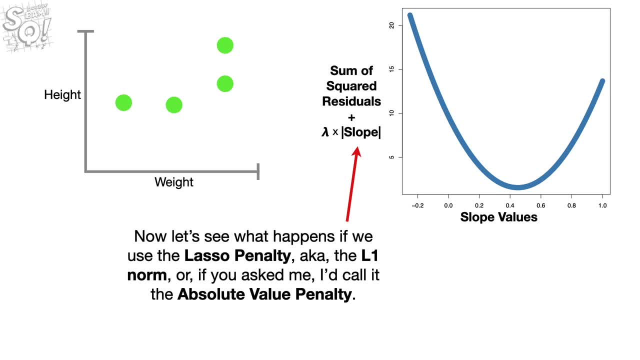 or, if you asked me, I'd call it the absolute value penalty. Unfortunately, no one asked me. Again, the thick blue line represents lambda equals 0, so there is no extra penalty. This is because when we plug lambda equals 0 into the equation, 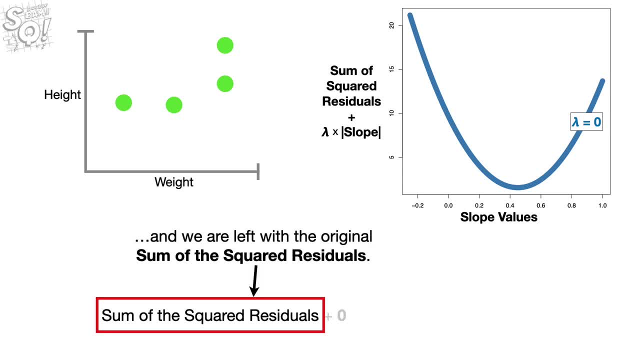 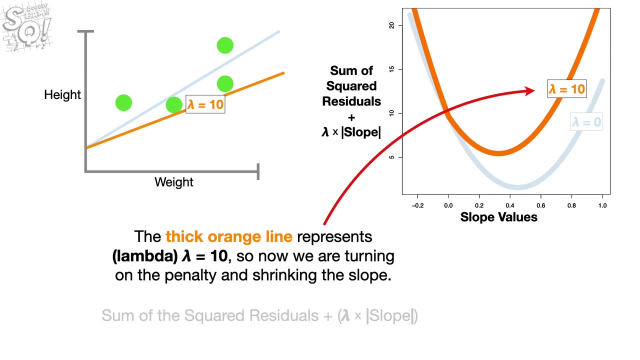 the penalty becomes 0.. And we are left with the original sum of the squared residuals. Just like before, we'll keep track of the best fitting line plus penalty. in this graph on the left, The thick orange line represents lambda equals 10,. 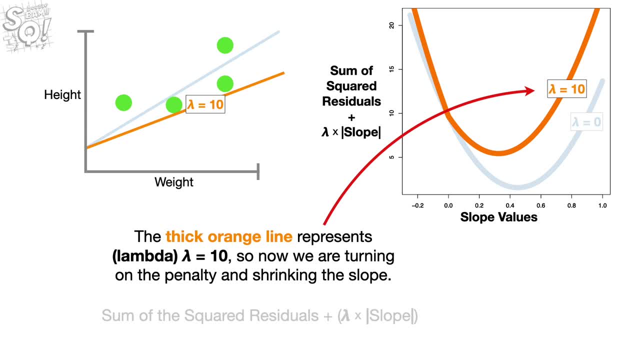 so now we are turning on the penalty and shrinking the slope. When lambda equals 10, we start to see a kink in the curve where the slope is 0. The thick green line represents lambda equals 20, and this kink at 0 is becoming more prominent. 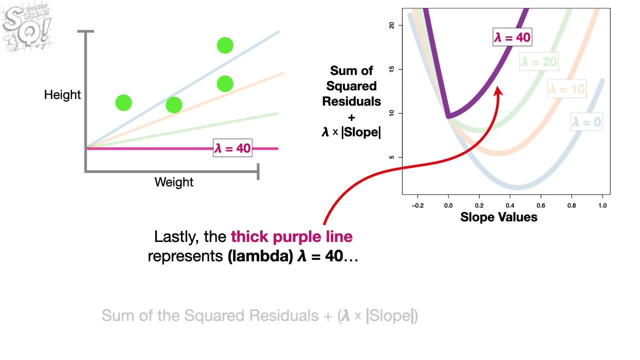 Lastly, the thick purple line represents lambda equals 40, and now the kink at 0 is super obvious. Now the lowest point in the purple curve, aka the optimal slope, given the absolute value penalty when lambda equals 40 is 0. 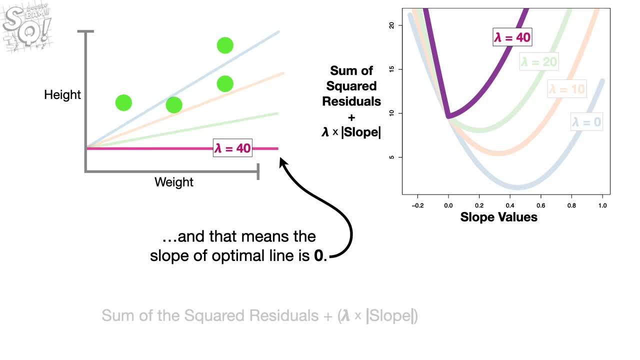 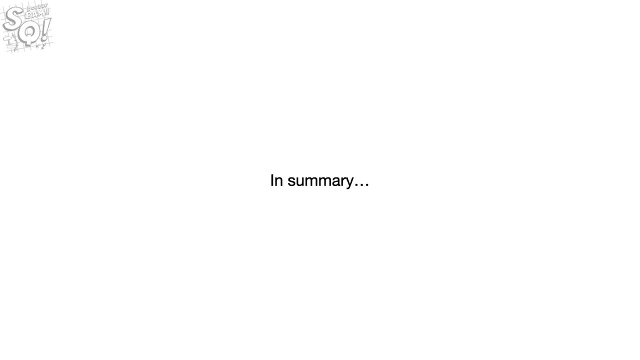 And that means the slope of the optimal line is 0.. And that means when lambda equals 40, we ignore weight as a variable when predicting height. Double bam, In summary, when we increase the ridge regression penalty, aka the L2 penalty. 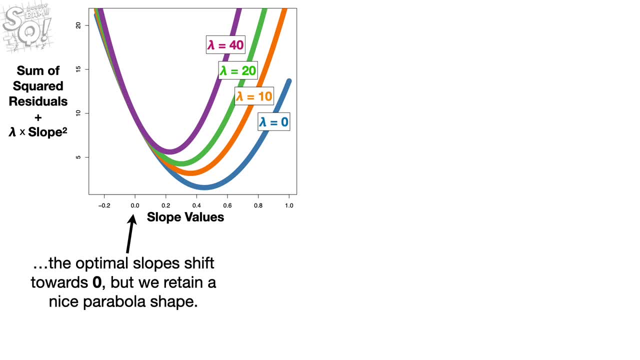 aka the square penalty. the optimal slopes shift towards 0, but we retain a nice parabola shape And even when we set lambda to something crazy high like 400,, we still end up with an optimal value greater than 0.. In contrast,